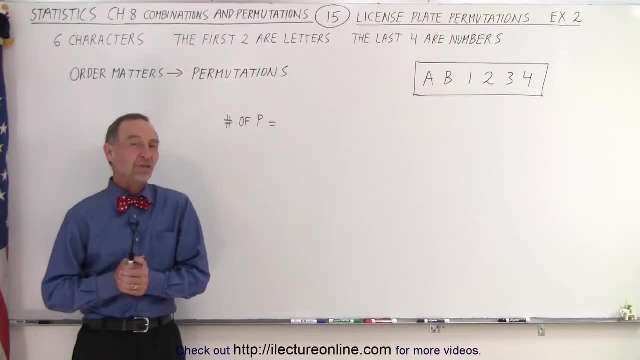 Welcome to our lecture online. What if we change the technique on putting together a license plate with six characters to make it more readable, And so we're going to restrict the first two characters to letters only and the last six characters to numbers only? Remember when it. 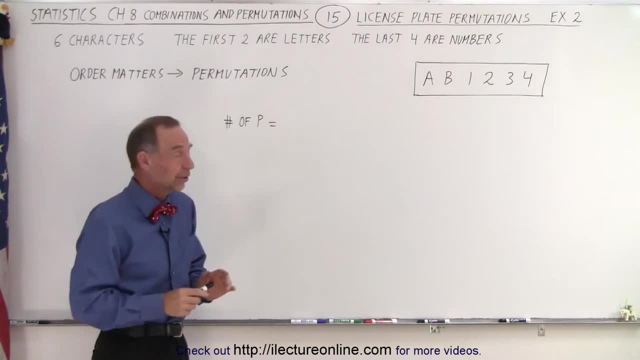 could have been anything. for all of the six characters, numbers or letters, we had over two billion permutations, So let's see how that changes. So the number of permutations can be picked by looking at that and saying okay to pick the number of permutations for one letter. 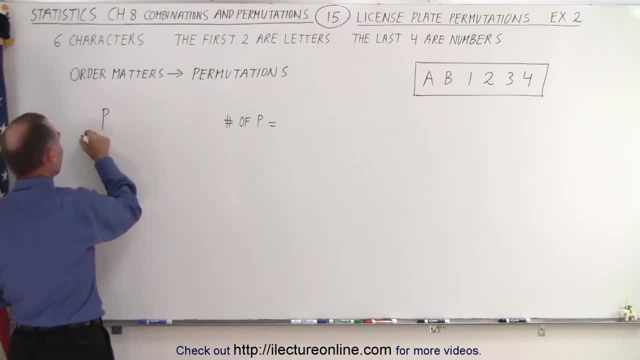 or one number. it'd be the permutation of nr and by definition this is equal to n factorial divided by n minus r factorial. And again, just because we picked a particular letter or a particular number, that letter or number can appear again, so it doesn't restrict the number. 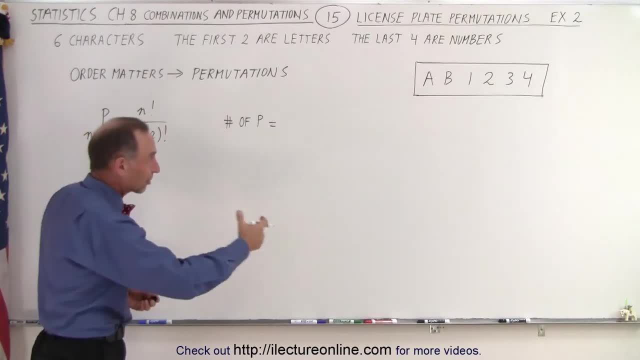 of letters or numbers we can choose from for the next characters we're choosing. So that means that this will be the case for every one of them And in the case of letters, for a letter that will become equal to. so this would be equal to: arrow there n factorial. 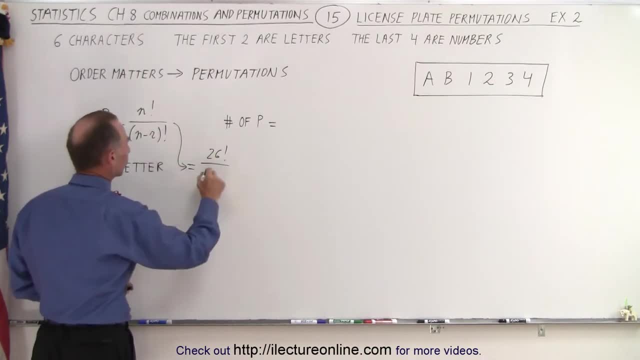 there's 26 letters divided by 26 minus 1, 26 minus 1 factorial, so this would be equal to 26.. And for numbers, that would be equal to 10 factorial divided by 10 minus 1 factorial, which is 10 factorial divided. 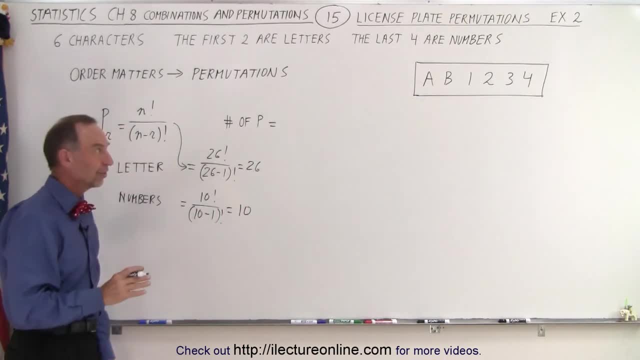 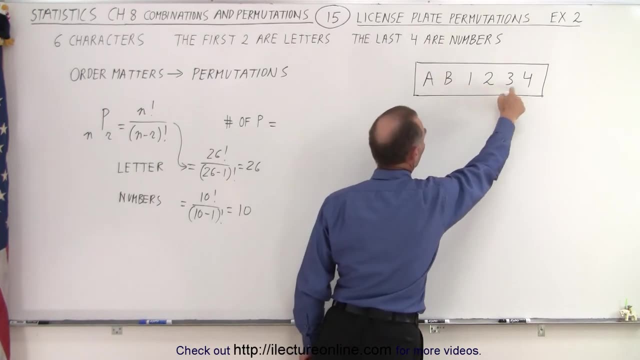 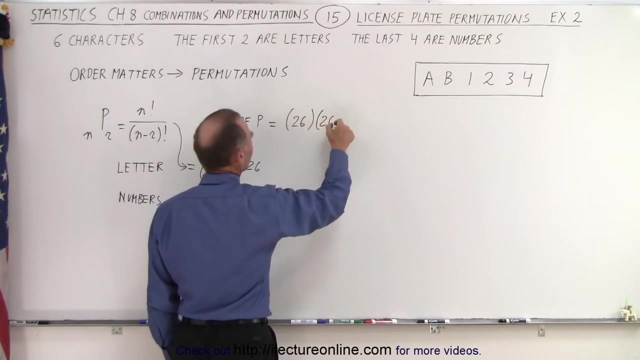 by 9 factorial, or simply 10.. And so you can see that the number of permutations for this character or this character is 26 for each, and the number of permutations for each of the numbers is just 10.. And so that becomes equal to 26 times 26 times 10,. 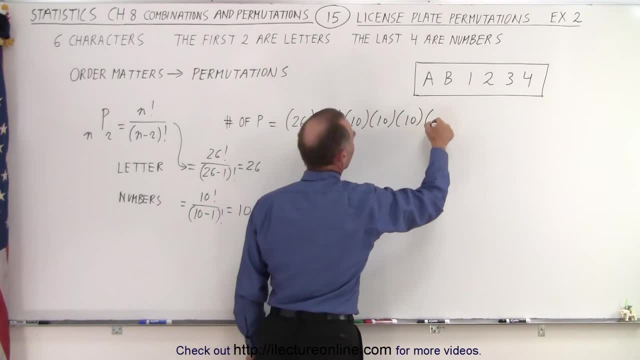 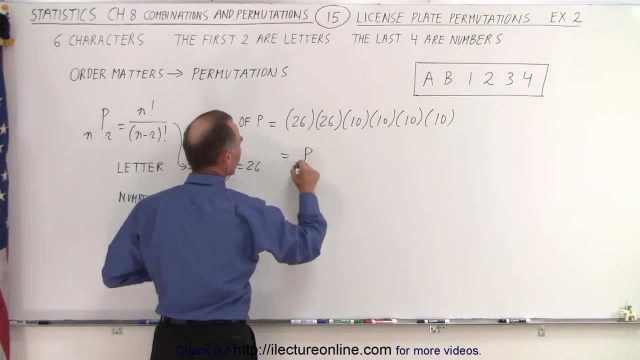 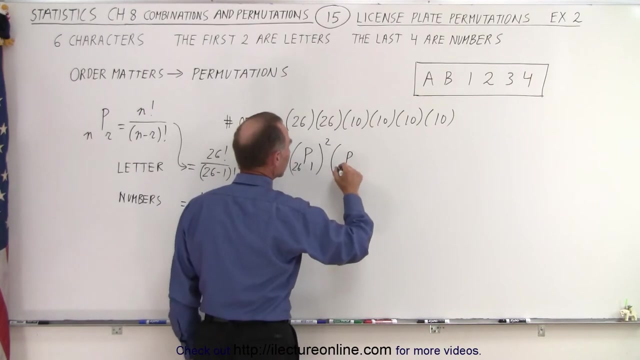 times 10, times 10, and times 10.. Or essentially this is equal to what we could put right here. so say p 26: 1 to the second power, times p 10, 1 to the fourth power, because this is essentially.